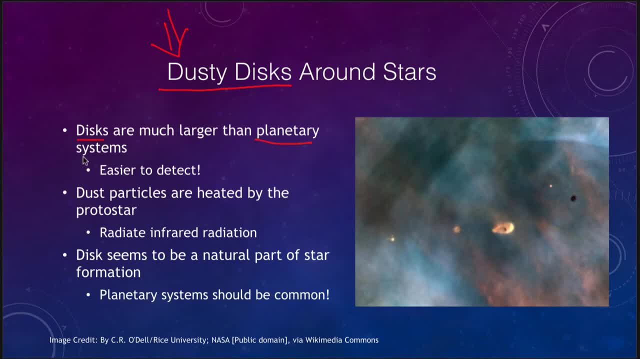 Now the idea is that these disks are much larger than the planetary systems themselves, making them easier to detect. So the dust particles are going to be heated up by the protostars And they're going to be radiating infrared radiation. So when we look, we see these little 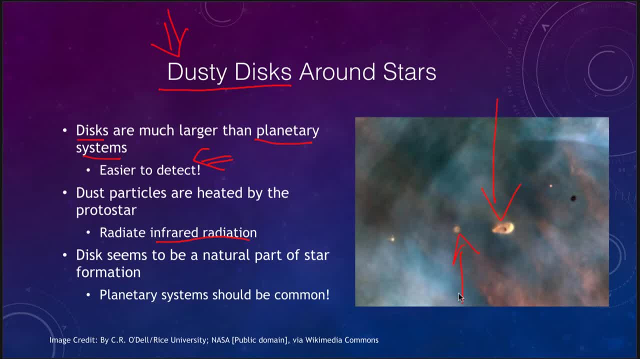 dusty areas, which are likely the beginnings of planetary systems that are forming, And when we look at star forming regions, the disk seems to be a natural part of star formation, meaning that there should be lots of planetary systems out there. How long does this process? 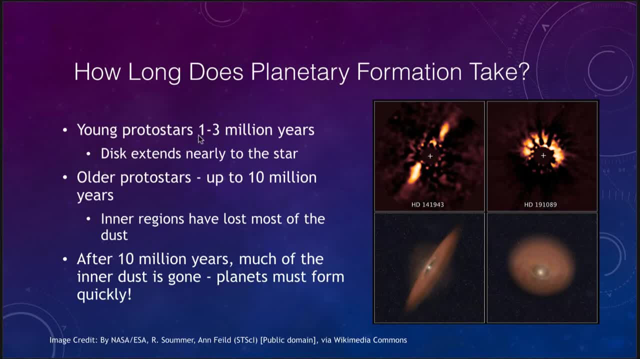 take, Well, a young protostar. Young protostars will live a couple million years and the disk will extend nearly into the star. So we can see some examples here where the star has been blocked out at the center and we can see the dusty disk around it. It's all a matter of the orientation with 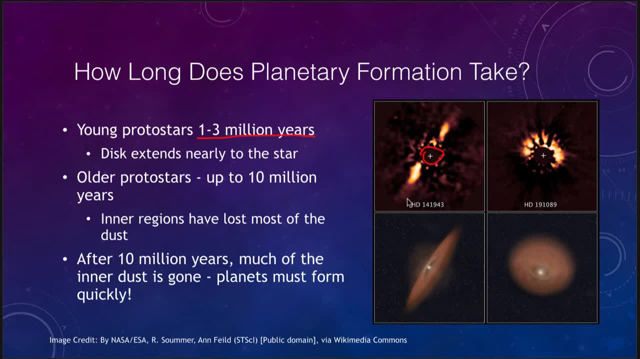 which we see them as well. So here we're looking at one close to edge on and you can see that the disk kind of runs diagonally across this. Here we're tilted a little bit more, looking at it more face on, and we can see the disk a little more surrounding the star. Now we 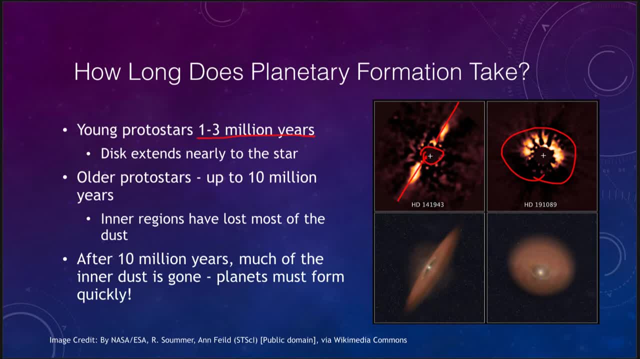 do have to block out the star, because the star is emitting far more light than the disk itself And that would mean that if we had the star in there it would be overwhelmingly bright. But we can get an idea with the artist conception sketches that we see down below. 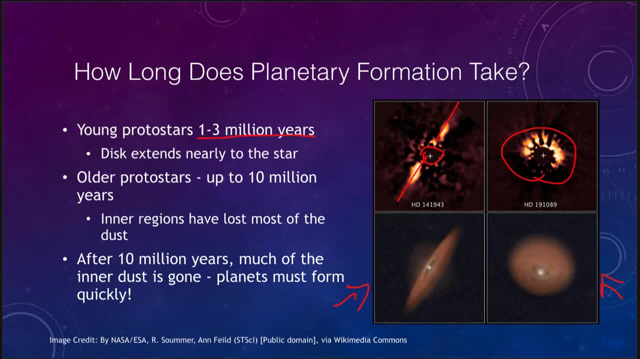 as to what these systems might look like. So let's take a look at the artist conception sketches that we see down below as to what these systems might look like. So let's take a look at the artist conception sketches that we see down below as to what these systems might look like. 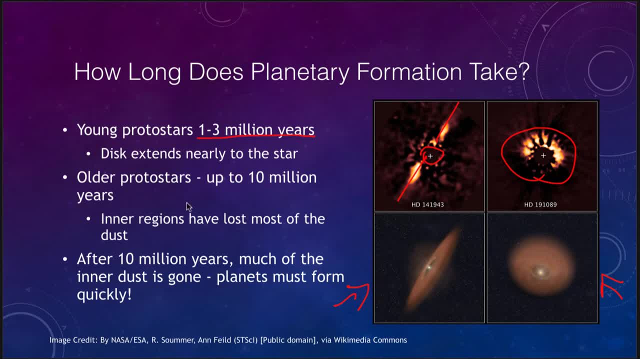 So in some of the older protostars, what we begin to see, even when we get up to 10 million years old, when they're very young, the disk extends nearly into the star. In older protostars, as they get older, the inner regions have lost most of their dust. So these intersections 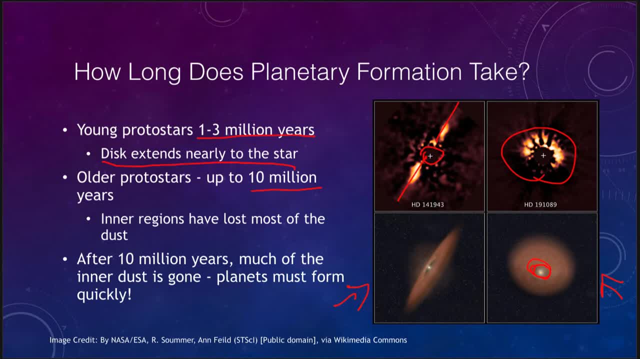 here are beginning to be cleared out by the material. So this must happen very quickly, because after about 10 million years that means the dust is gone, The material that could possibly build the planets is gone, So the star formation must have formed within this 10 million year time frame. 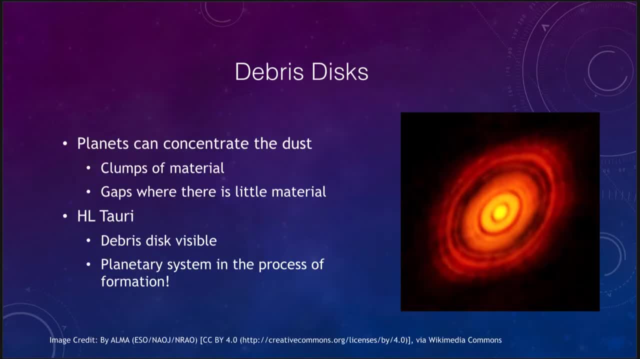 Now, when we look at some of these, we can also see disks of debris around the material. We get various clumps of material where dust can be concentrated, So we're going to start seeing things like the rings that we see around some of the planets. 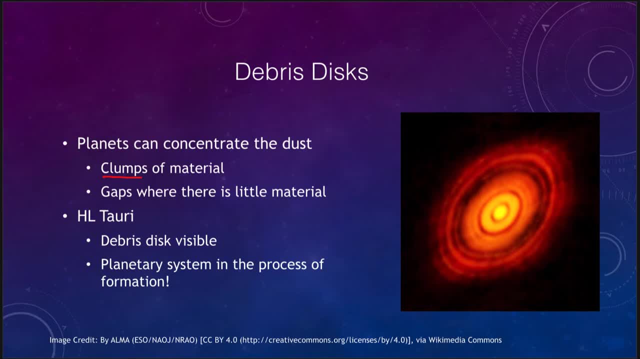 We get denser areas and less dense areas within the disk of material. So there are various gaps where there's little material and clumps where there is more material, And we see HL Tori as one example where we can see this debris disk We can actually see. 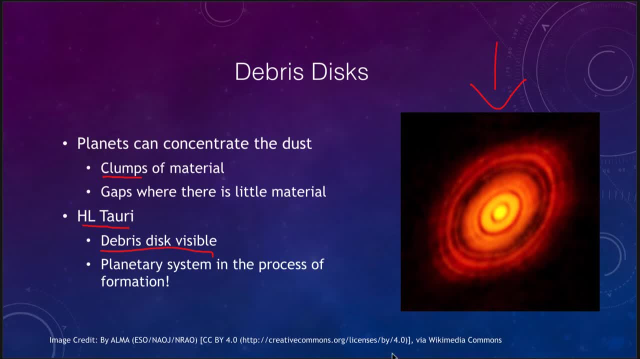 this in the infrared portion of the spectrum and we see the protostar at the center and then the different rings of material And very likely, within each of these rings we are beginning to see the beginnings of the formation of a planetary system. So what are some of the methods that we can search for actual exoplanets? Here we're seeing 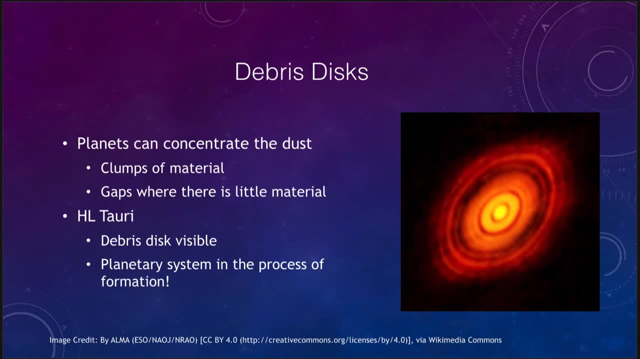 the beginnings of their formation, and we've known about this for a few decades. It's only been in the last 25 years or so that we've begun to detect extrasolar planets, planets outside our solar system. So what are some of the methods that we're going to look at? 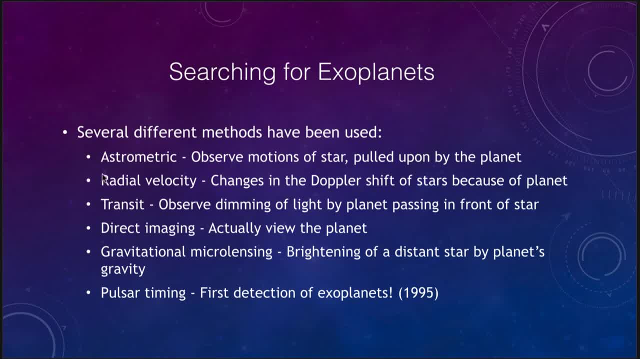 These we will talk about in a little bit more detail over the course of this lecture. There is the astrometric method, where we look at the motions of the star and how the position of the star changes. We can look at the radial velocity method, where we look at changes in 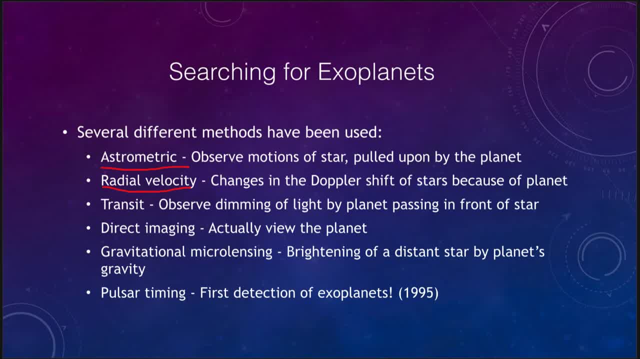 the Doppler shift of the star, So the velocity of the star changes. It's similar to the astrometric method, except here we're looking at position, Here we're looking at velocity. We can look at the astrometric method where we observe the dimming of the light when a planet passes. 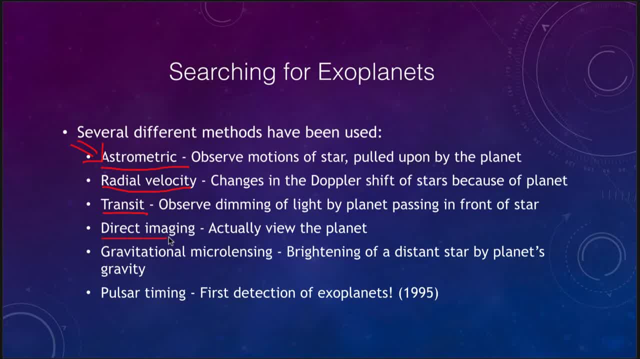 in front of the star And, a little more rare, we can see direct imaging, where we actually can view the planet. We can actually see the light from the planet And a couple of less common methods: gravitational microlensing When the planet's planet passes directly in. 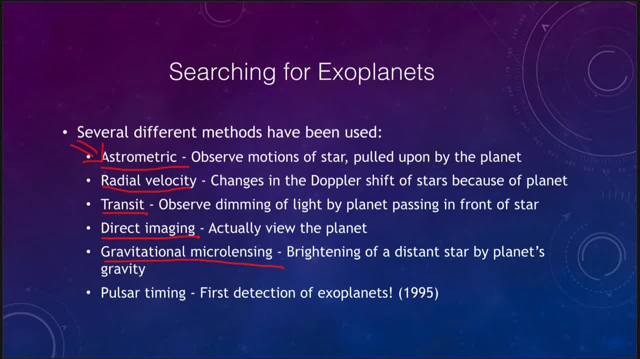 front of a distant star- not the one it's orbiting, but in front of another star. it'll brighten that star and cause it to temporarily increase, And that allows us to detect the planet that way. And finally, a last one that I really 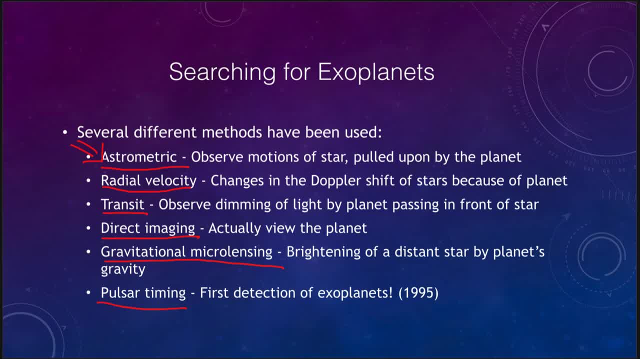 won't go into any more detail on. in is pulsar timing. Variations in the timing of the pulsar can imply that there are planets orbiting it, tugging on the pulsar. This was actually the first detection of exoplanets back in the 1990s, The first detection of planets. 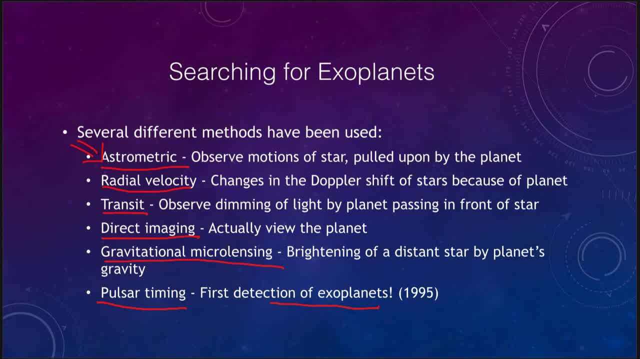 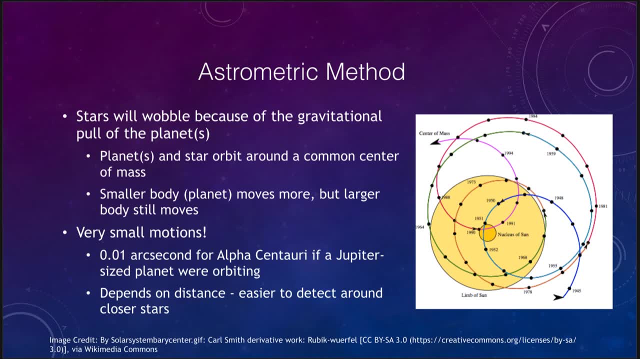 outside our solar system. So let's look at some of these methods, And first we want to look at the astrometric method. What happens is that stars will wobble because the planets are pulling on them. In reality, we talk about a planet orbiting around. 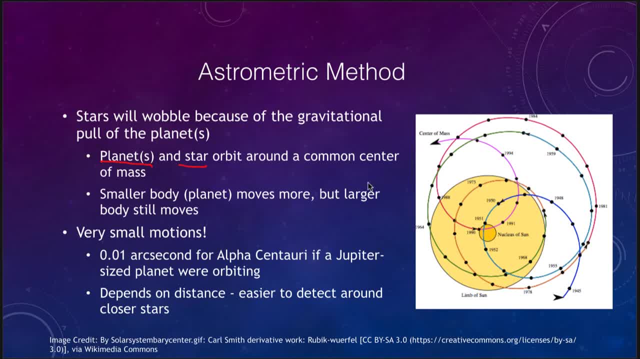 a star So, but in reality they orbit around a common center of mass. So really the planet orbits and the star orbits as well, Just that the stars orbit is often within the star. often that center of mass is actually within the star itself, And the image we see here shows where the center of 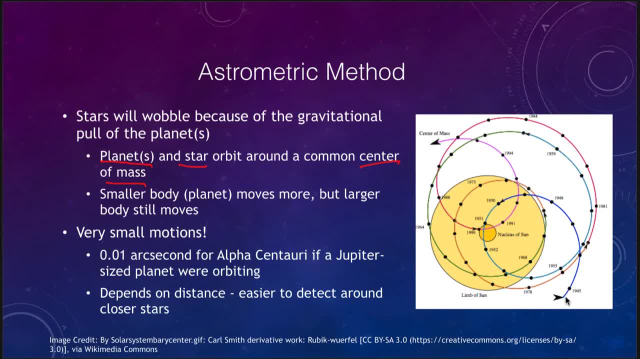 mass of the solar system is. Sometimes it is outside the sun by a little bit, And other times it is actually deep inside the sun. it depends on the relative positioning of the planets at the time. So what we would see with this is that we're depending on where. 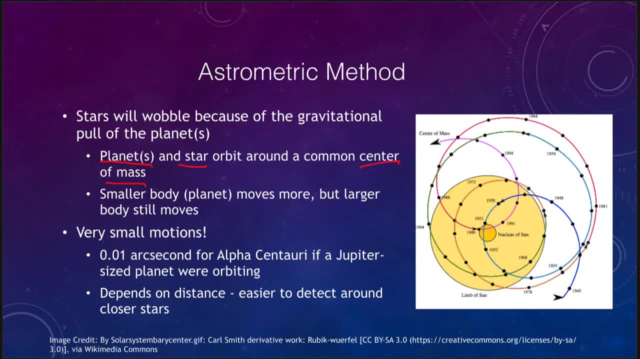 that center of mass is. the sun would be moving more or less, And some distant astronomer would be able to see the sun wobbling a little bit in its position. You would be able to see its position change. So while the smaller body moves more, the larger body, the star, still does. 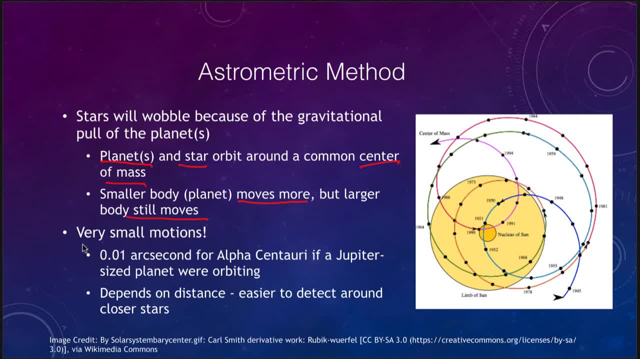 move and that is something that can be detected. However, it is extremely small and difficult to detect For Alpha Centauri, the nearest star to us. if we had a Jupiter sized planet orbiting it, that would give a shift of 0.01. 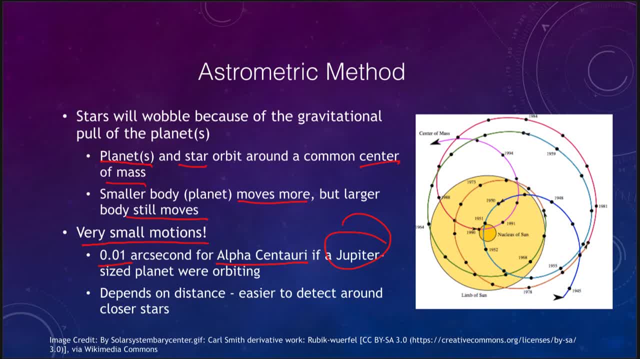 arcsecond. Now, that's definitely detectable. we can detect even smaller motions than that, but it's extremely small and this is for the nearest stars. If it gets a little further away, it's going to be harder and harder to detect these motions and they will be able to be detected with less accuracy, And this 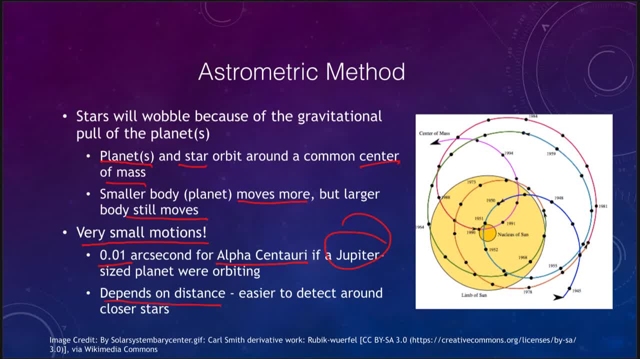 also, again, significantly depends on distance, Because it's going, the motions are going to be easier to detect if the star is close to us than if it is further away. So astrometric method is one used. One of the more common ones that we use is: 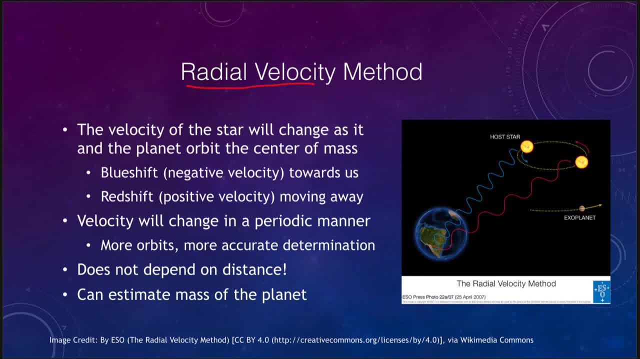 what we call the radial velocity method. What happens? here again, we're looking at the same kind of thing we talked about for the astrometric method. In reality, the star is actually orbiting as well. So the star orbits around the center of 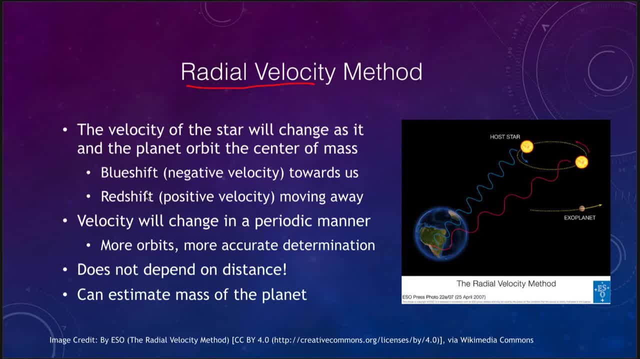 mass based on the exoplanets motion, And when the star is moving towards us, it is blue shifted, which we call given negative velocity. When it is moving away from us, it's a redshift, or what we call a positive velocity. So, as the star orbits, at some point it's moving in the direction of 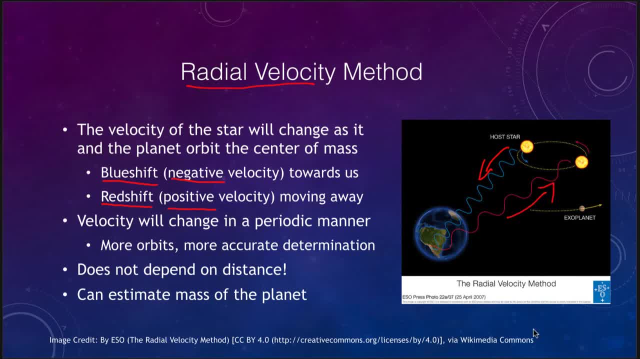 the earth and we will see a blue shift. A little while later, we will see a redshift. Now, the period of the motion is exactly the same as that of the planet, So if this planet takes one year to orbit, so will the star. So we would see a blue. 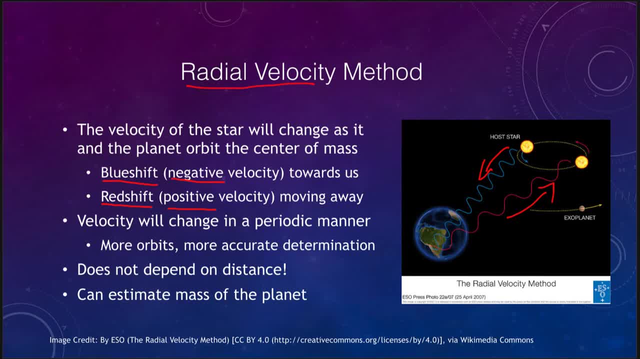 shift and six months later we would see a redshift for something that took one year to orbit. So there will be a periodic change in this. Now, the more orbits we can get, the more accurate the determination. So just seeing one orbit may give us a hint that. 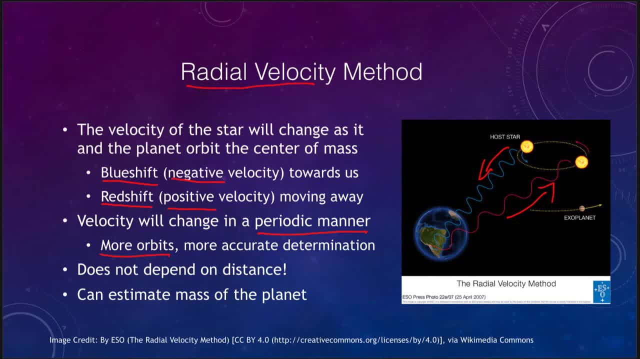 a planet is there, but may not be enough for confirmation. We need to get more and more orbits, and that's why it's easier to detect closer planets to their stars, because they orbit faster and they were able to see this quicker, In just a few. 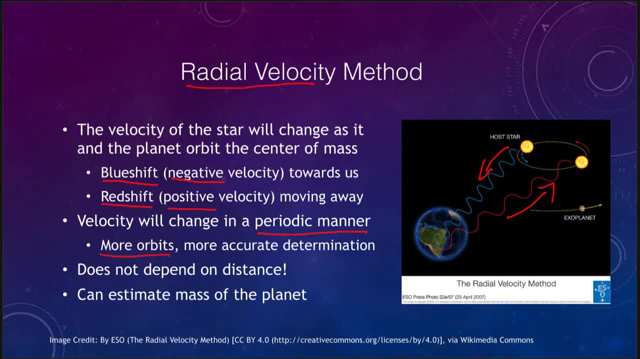 years, we can get several orbits, Whereas a planet like Jupiter, which takes 12 years to orbit, would take decades. The key about this one is that it does not depend on the distance. All we need to see is the star, and all we need to do is to measure the Doppler. 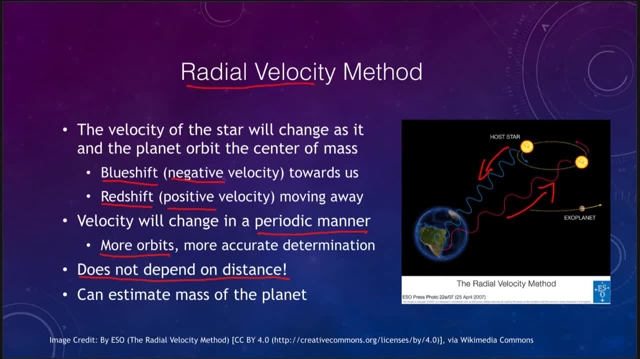 shift of the star, So all we need to do is to take its spectrum. It does not. as long as we can see the star, it does not matter. So this does not depend on the distance, as long as it's not so far away that we cannot see the star. And it does. 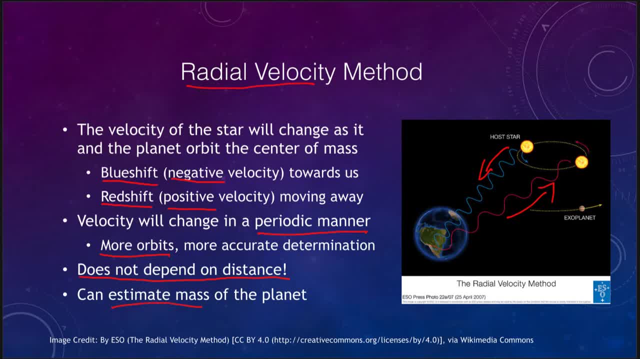 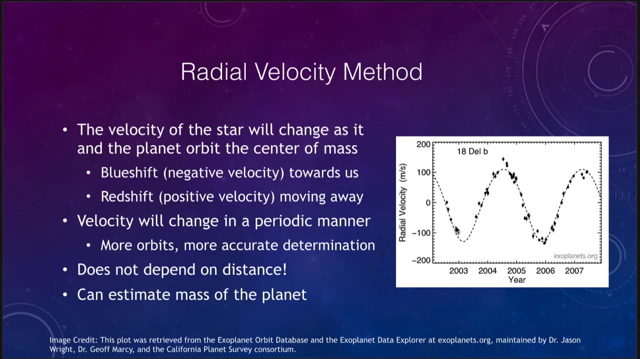 allow us to estimate the mass of the planet based on the motions of the star itself. Now, when we can see this, what we get in terms of data that we see? if we look at an example of one of these, we see that the star will vary in velocity. We will get a negative. 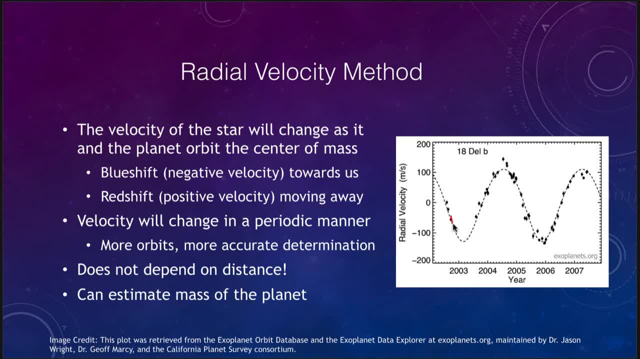 velocity when it's moving towards us down here, and then a positive velocity when it's moving away. So we'll see this constant change and we can fit that with a little periodic curve here And then allow that to determine the amount of the shift, the amount of the. 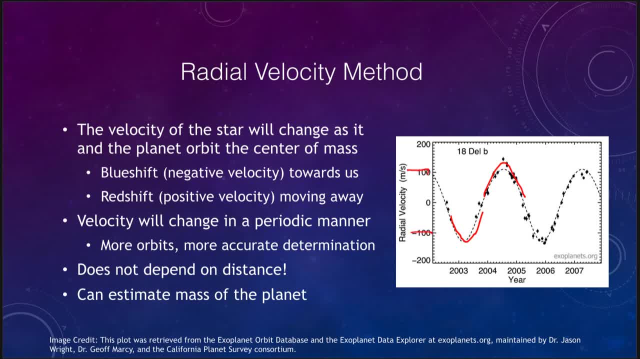 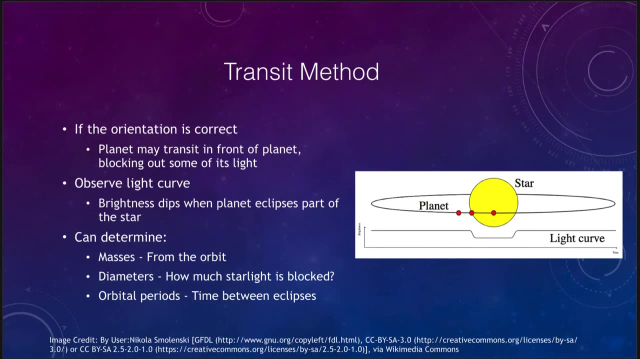 velocity change will allow you to determine the mass of the planet. So we can actually determine some of the properties of this based on these types of observations. Now, one of the more common we used- radial velocity is one, but the other common method used is called the transit method, The transit, 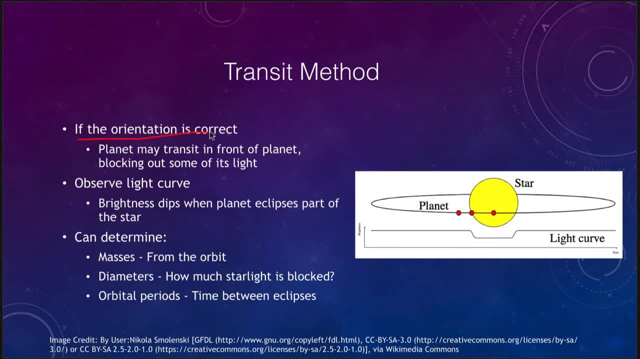 method works only if the orientation of the system is correct, Meaning that it has to be almost seen edge on. You can imagine you see it here almost completely edge on, and the planet passes in front of the star and will temporarily dim its light. So if we look at what we call the light curve, we see 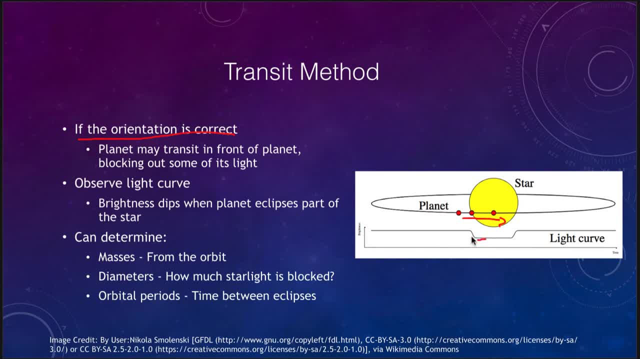 the brightness here and when the planet passes in front of the star it dims off a little bit of that light. So a little bit of the light is missing from the star and it looks a little bit dimmer. So when we observe this, we will see the planet eclipsing part of the star and we will see that. 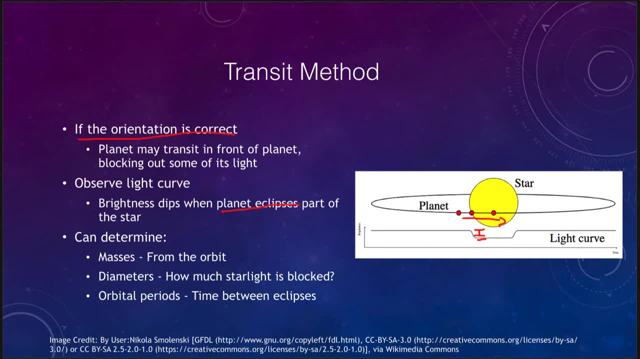 light curve, drop down in brightness And what we can determine here is the mass of the planet from the orbit and the diameters, the size and the orbital periods. So we can get an idea a little bit more about that if we look at this. 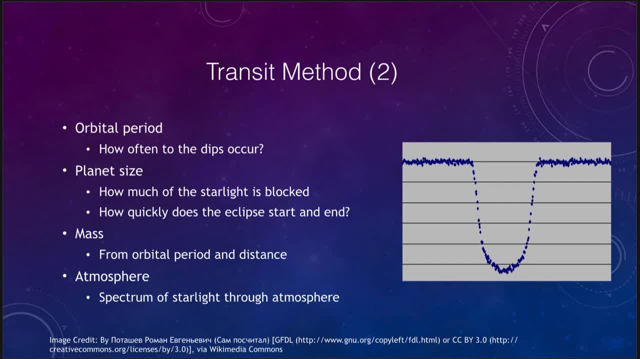 image. Here is a little more detailed light curve that we might see- And we can use that to really be able to determine a lot of this- by how often the dips occur. If they occur every once every year, then the orbital period is one year. If they occur every, 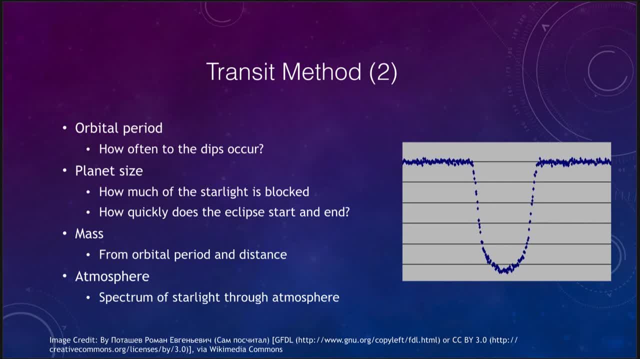 five days, then the orbital period is five days. So that tells us how often the planet passes in front of the star For the earth. the earth would pass in front of the sun for an object for a distant astronomy, once every year. Jupiter would be. 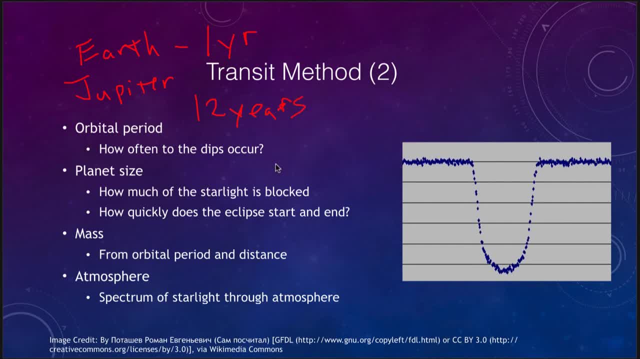 every ten times 12 years. So how often it happens depends on the orbital period, The planet size we can learn from how much of the starlight is blocked. So how much does this dip down during the eclipse? And we can also get an idea by how quickly. 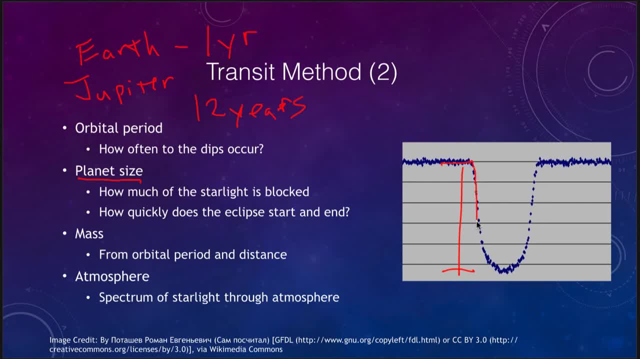 the eclipse starts and ends, How quickly does that planet get in front of the star? And the very faster it occurs, the steeper this is. then the planet is much smaller. If it gets into an eclipse and comes out very quickly, then it's a very, very, very small planet. 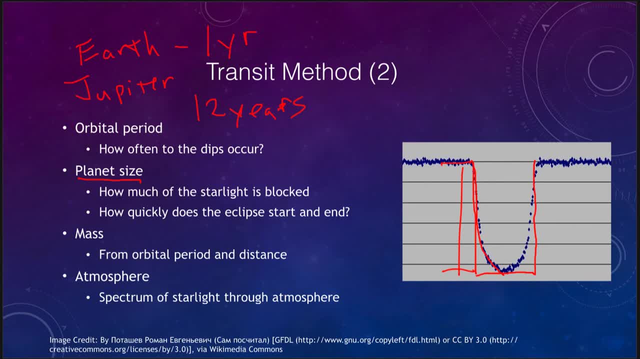 because it doesn't take it long to block the star. A very large planet will take more time to slowly get its body in front of the star. We can determine the mass from the orbital period and the distance. So once we determine those, then we 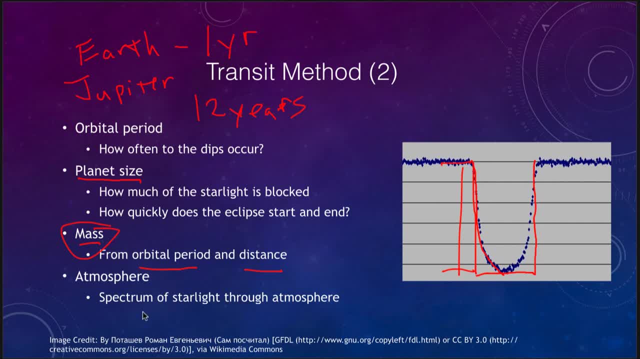 can get ideas of the mass looking at all of this, And we may even be able To determine something about an atmosphere by looking at the starlight when it's going through that atmosphere. It will absorb various lines depending on its composition, And we'll be able to allow us then. 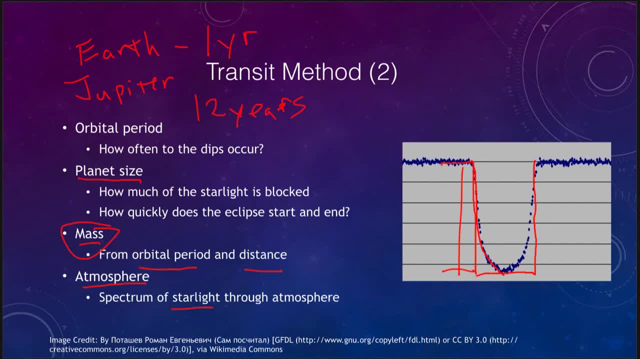 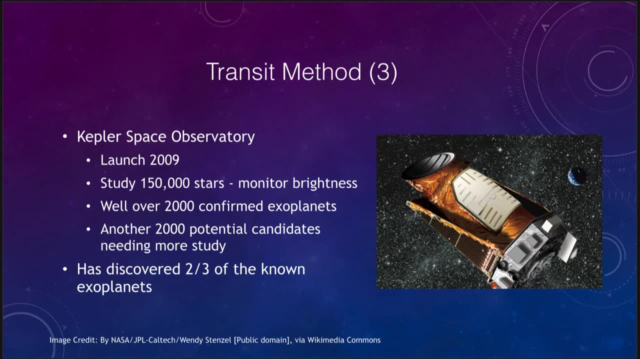 to determine a little bit about what the composition of that is. Now, the key for the transit method has been the Kepler Space Observatory That was launched in 2000.. And the Kepler Space Observatory was launched in 2009 and studies 150,000 stars in a small portion of the sky. 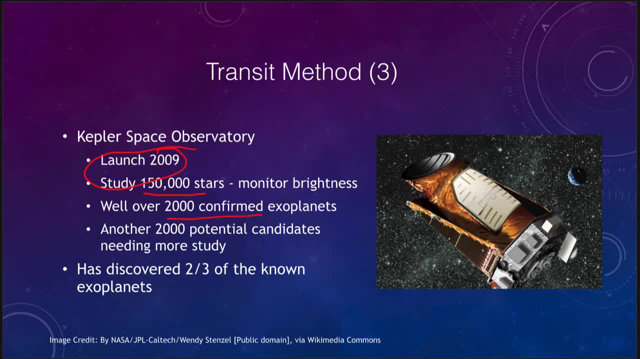 It has now confirmed over 2,000 exoplanets. So a large percentage of the exoplanets that have been discovered so far have been discovered by this satellite, And there are 2,000 more that are potential candidates that need additional study. 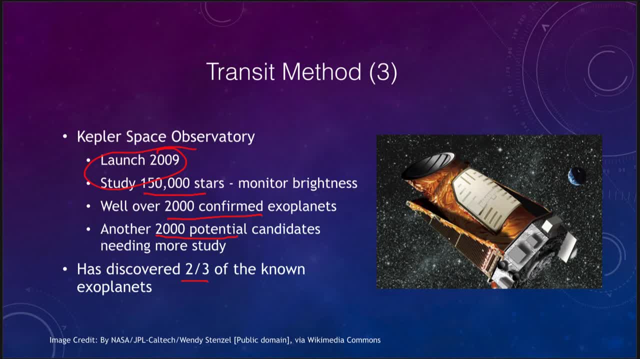 At this point, it's discovered 2 thirds of the known exoplanets And we're able to see that the stars are actually orbiting the stars over and over again, measuring their brightness and watching for those little dips that signify that a planet has. 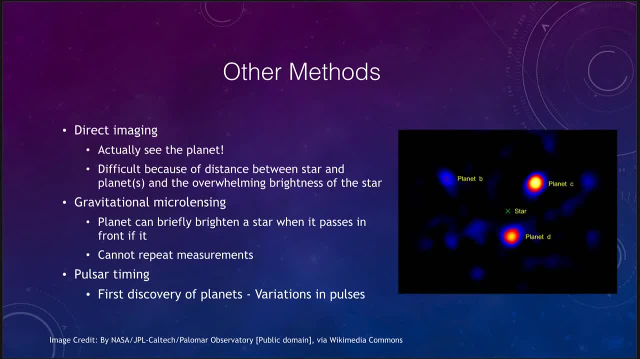 passed in front of the star. Now some of the other methods that we can use, in addition to these more common ones, are direct imaging. So if we block out the starlight and look here in the infrared, we can actually see the planets. 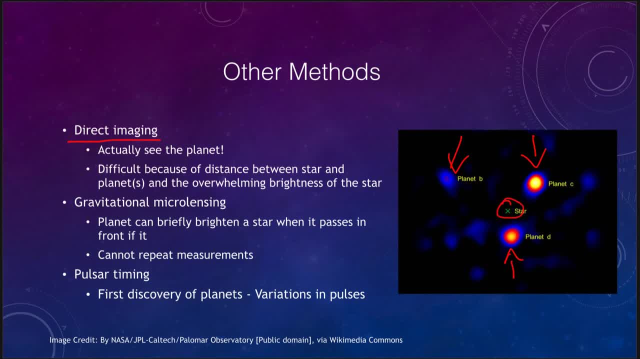 So we can see several planets here that would actually be present here, but we're not looking at a wavelength where the star would be easily visible, but where the planets are. In these cases, we are just seeing the light from the planet. Any time you see a sketch of what an exoplanet looks like. 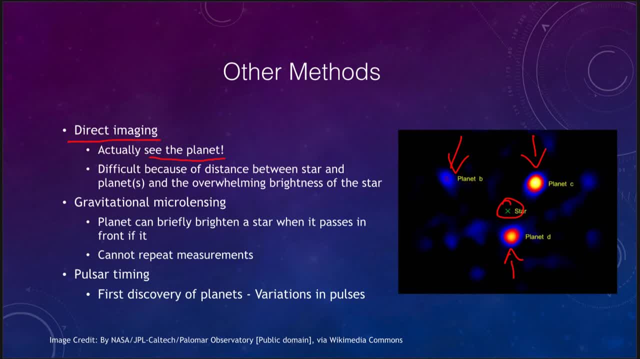 it is always an artist's conception. We cannot actually see any of these planets other than the fact that they exist in their light. But this is difficult because the planets are often very close to their star And the star is always there, And the star is always there. 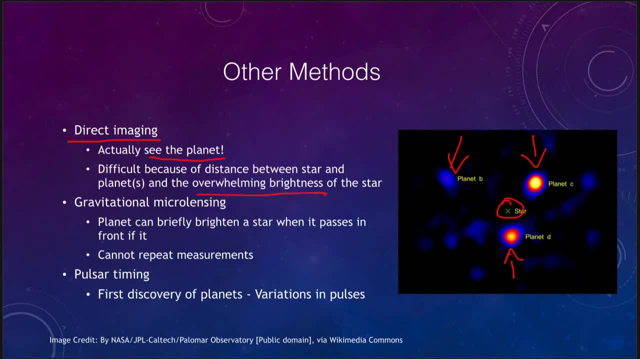 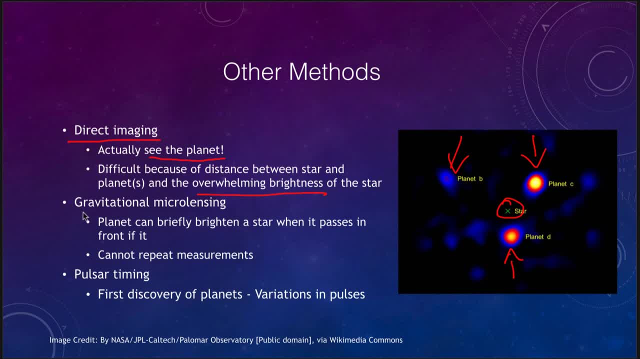 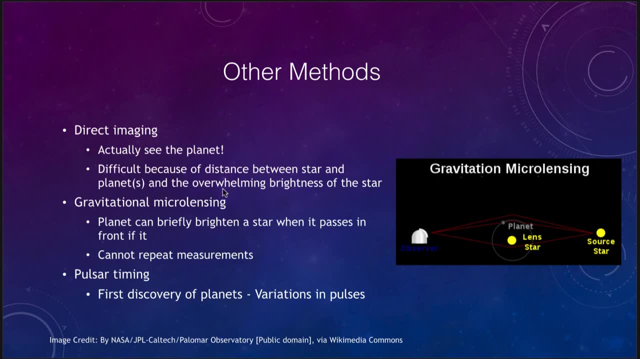 direct imaging of exoplanets. Gravitational microlensing is another method that is used And that is done here, And what happens is that a planet can briefly make a star appear brighter when it passes in front of it, So the star can cause it to lens. 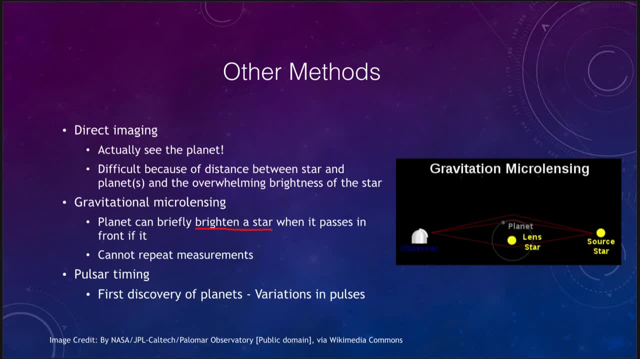 and a planet can cause it to lens a little bit more. Now, this is a nice way to be able to detect things that are further away from their star, because it does not depend on being close. The radial velocity method is a lot easier to do when things are closer to the star. 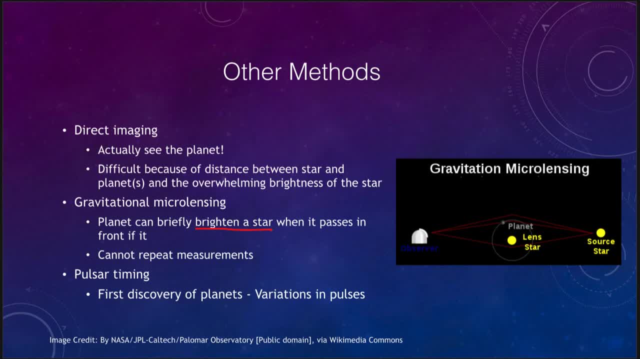 because they occur more often. The transits will occur more often for very small orbits. A microlensing can occur even if the orbit is very far away. Even a planet like Jupiter or Saturn or Uranus or Neptune could be detected through this method.